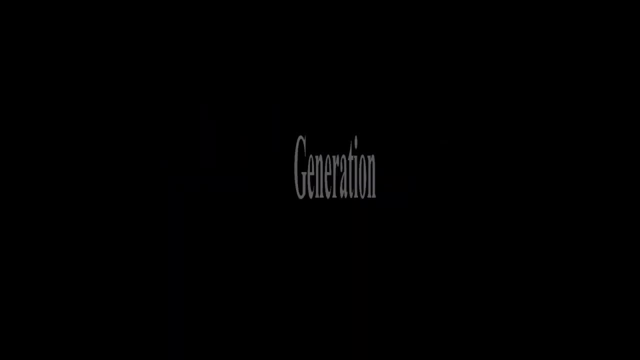 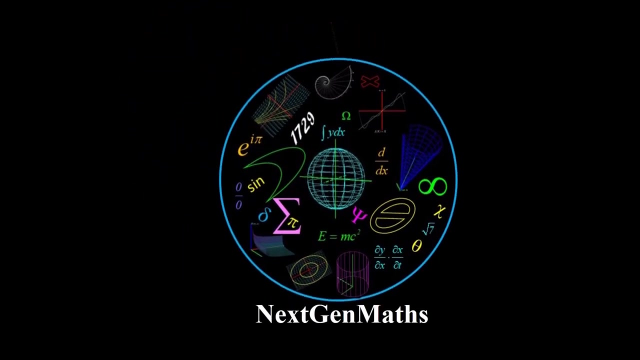 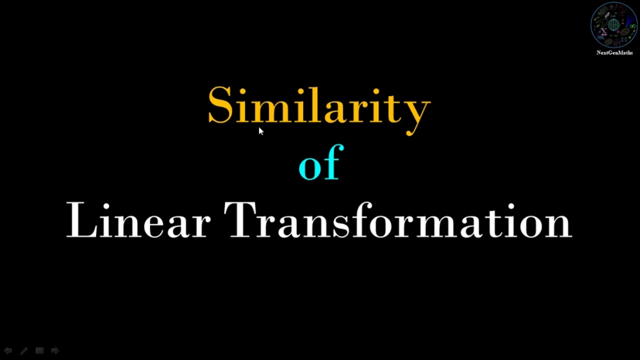 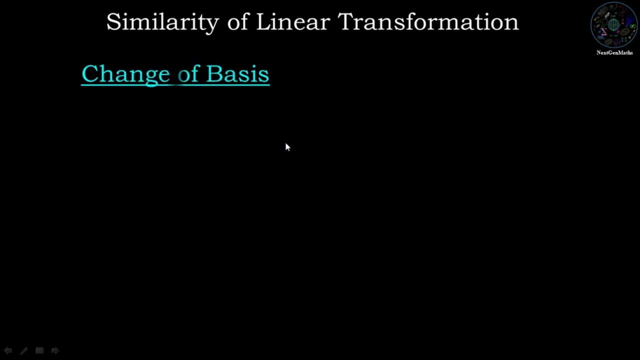 Hello friends, in this video we are going to discuss similarity of linear transformation. The similarity of linear transformation is extension of change of basis of linear transformation. So first we recall the concept of change of basis of linear transformation. So we considered the transformation I, V to V, where I is a identity linear transformation. 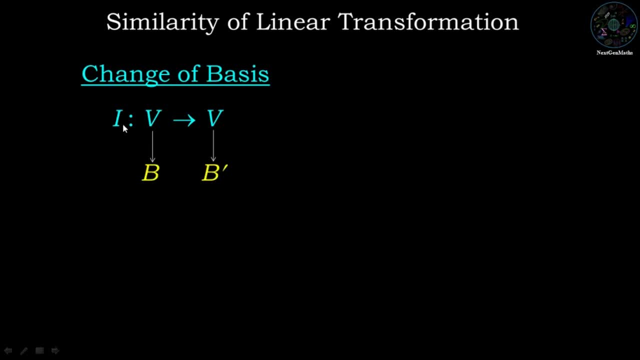 where domain has basis B and codomain has basis B'. So I is identity linear transformation. so I of V equal to V. The difference is that the image vector V as basis B' and the domain vector V as basis B. So this identity linear transformation will give the change of basis of vector space. 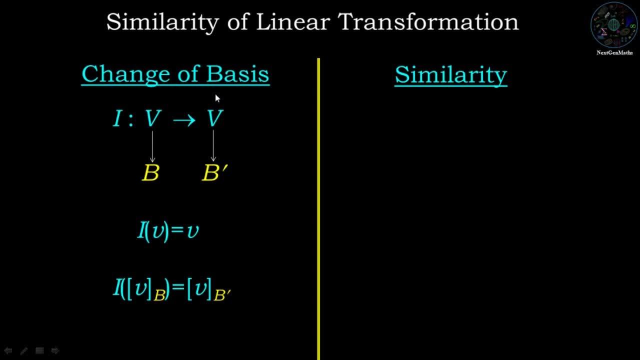 Now the similarity is extension of change of basis of linear transformation By changing I to the generalized linear transformation T, V to V, where domain has basis B and codomain has basis B' Suppose T of V equal to W, that means image of V under the linear transformation, T is 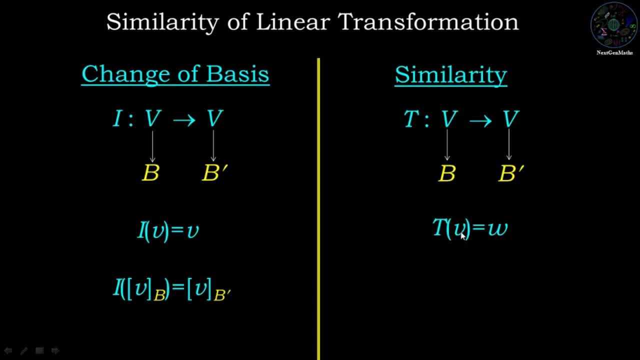 vector W. V is an element of domain and W is an element of codomain. Therefore T V be equal to W' W is equal to T V, therefore T V be equal to T V' So in the similarity we have two steps to get the image. 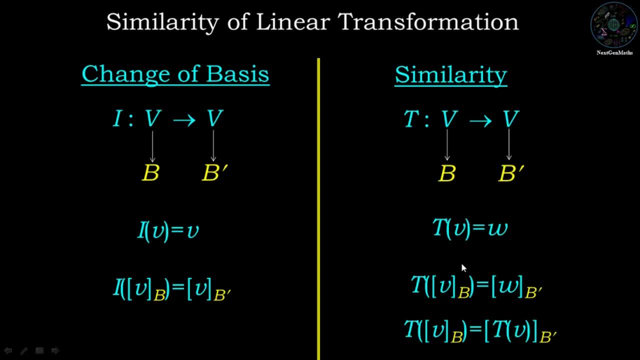 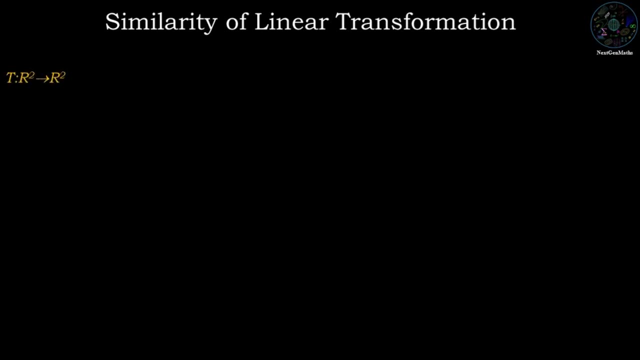 First step is change of basis and the second step is find the image. or first step is find the image And then change the basis. We are going to understand this process using one example. Suppose T is defined from R2 to R2, the domain has basis B equal to 1, 0, 0, 1 and the codomain 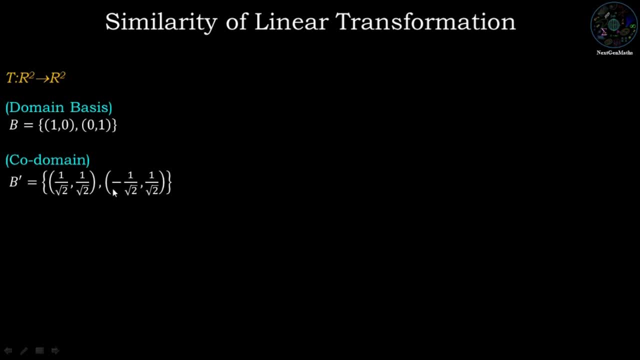 has basis B' is equal to 1 by root 2, 1 by root 2, minus 1 by root 2, plus 1 by root 2.. And the transformation is defined as Tx is equal to 2x. that means every vector double. 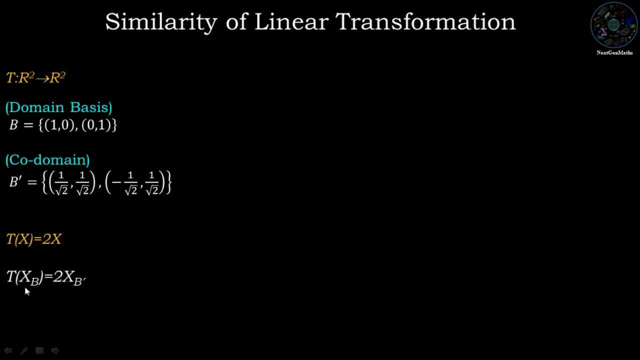 in its image. You can rewrite with respect to basis. so TxB is equal to 2 times xB'. So to get this xB' we have to follow two steps. First step is change of basis and then take the image, or first take the image and then 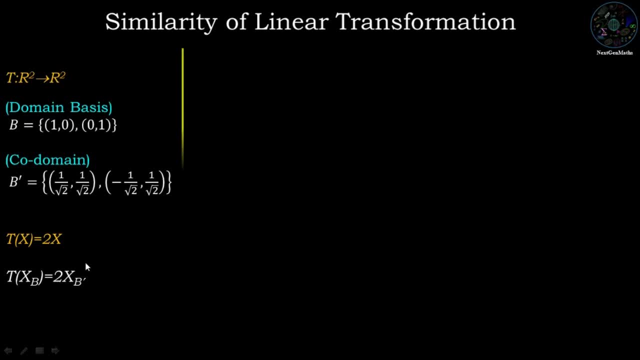 change the basis. We are going to understand the geometry. Suppose we have an ellipse in the domain B. Now we are going to find the image of this ellipse using this transformation: Tx is equal to 2x, So first we take the change of basis. 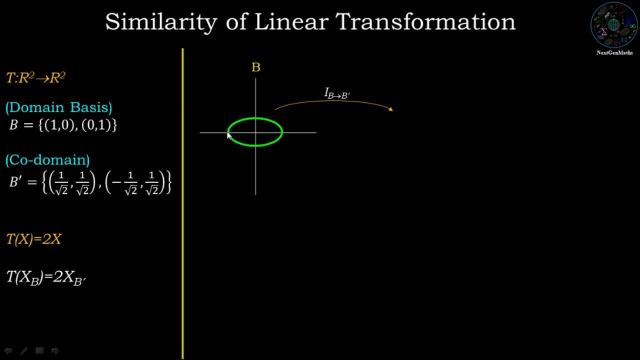 So by changing the basis B to B', this ellipse is now 2x. Transfer to the ellipse with the 45 degree rotation. Now we are going to take the image of ellipse. under this transformation, Tx is equal to 2x. then we have this: ellipse will double the original ellipse after the transformation. 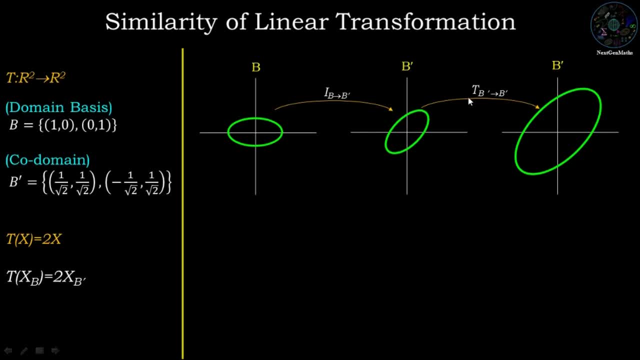 So, Therefore, To get the final result of ellipse, we have to do two transformation. one is identity transformation from B to B' and the second one is transformation T from B' to B' Now we are going to discuss the second path to get the image. 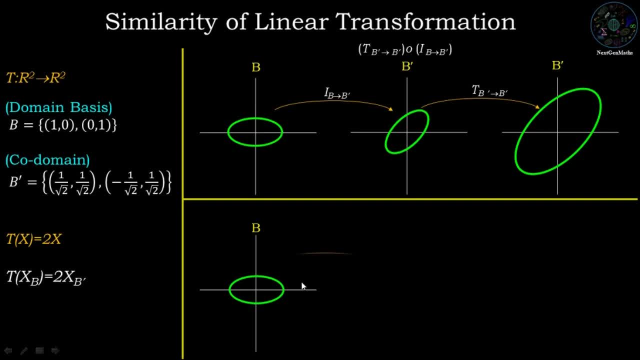 So we have ellipse in the domain. Now first we take the image, So image is double the original ellipse. Now we are going to take the image, So image is double the original image. Therefore it double the image. So it is a transformation T B to B'. 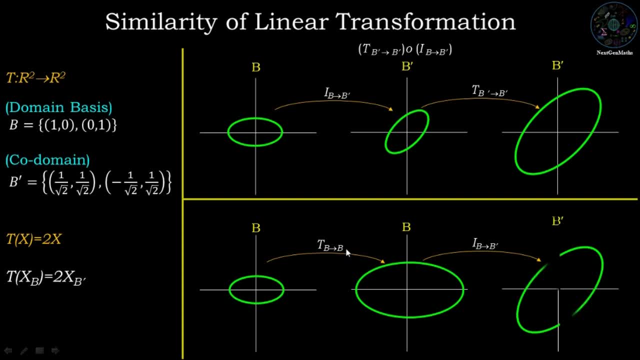 Now we change the basis and it is rotated by the 45 degree. So here we have transformation is a composition map of two transformation: T B to B' and I B to B' So in both the process We have the same result. So this process are called the similar linear transformation. 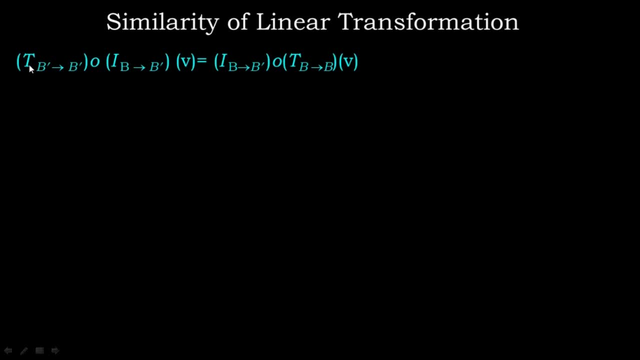 So this, two linear transformations: first, composition T B' to B' with I B to B' V, equal to I B to B' composed with T B to B V. So the matrix associated with this linear transformation, If P is a transition matrix, 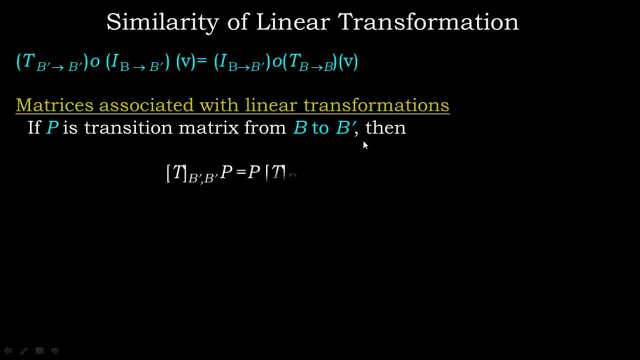 From B to B' then T B' B', P equal to P T B'. therefore you can rewrite T B' P equal to P T B' the notation T B' B' can be written as T B' and T B' written in the form of T. 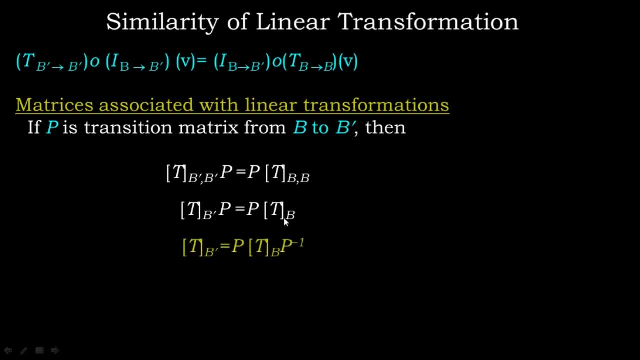 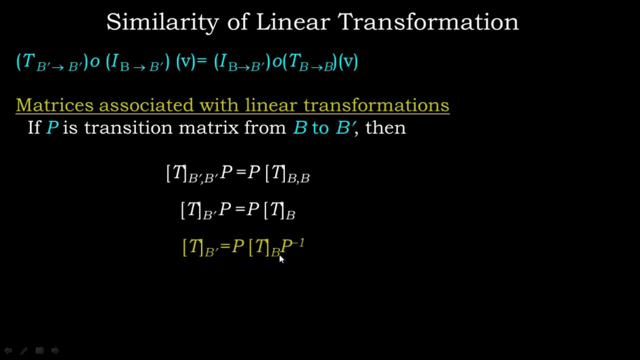 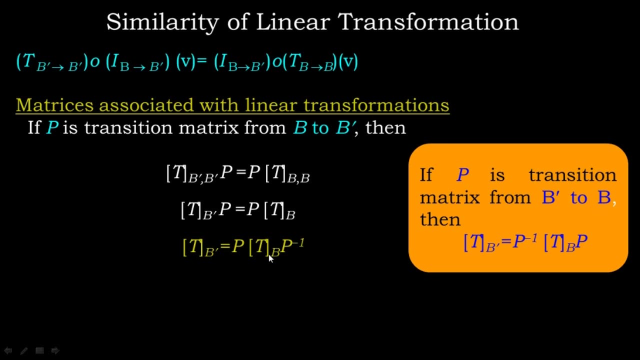 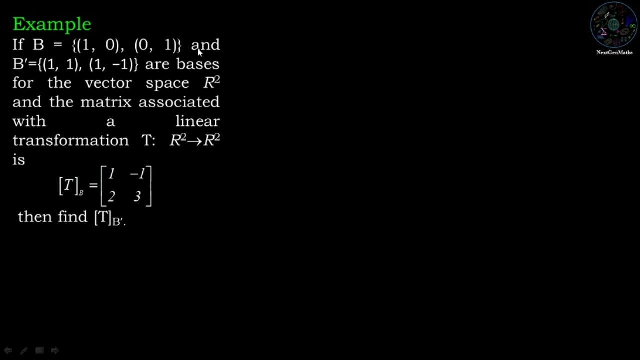 So therefore, this T B' and T B are called the similar matrices, where the transition matrix P from B to B' If you consider the transition matrix P from B' to B' then this result can be written in the form of T: B' equal to P inverse TbP. Now we are going to discuss one example. If B equal to 1, 0, 0, 1. 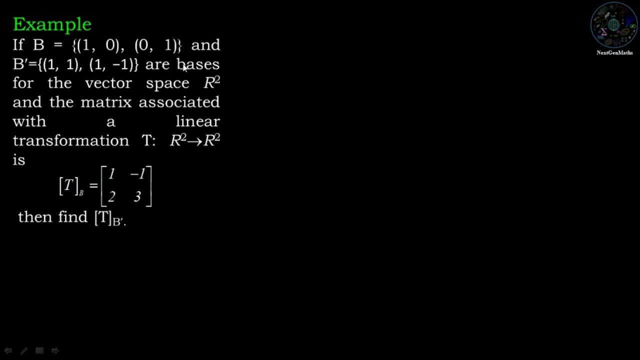 and B dash is equal to 1,, 1,, 1 minus 1 are basis for the vector space R2 and the matrix associated with the linear transformation T R2 to R2 is Tb equal to 1, minus 1,, 2, 3. then find Tb dash. 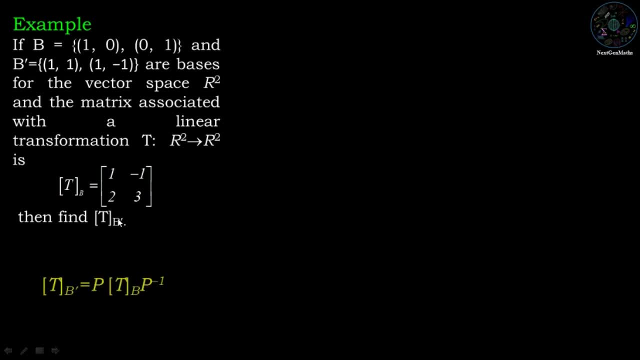 Now to solve this example, we will use the result. with Tb, dash is equal to P, Tb, P inverse. So for that we require transition matrix V1 equal to 1, 0, V2 equal to 0 and belongs to B, W1 equal to. 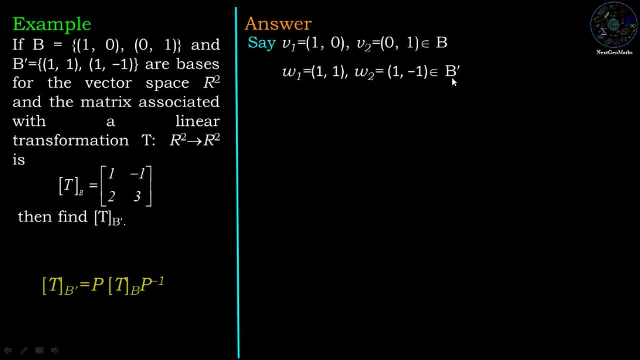 V2 equal to 0 and belongs to B 1, 1 and W2 equal to 1, minus 1 belongs to B dash. Now transition matrix P from B to B dash, Step 1, construction of augmented matrix B dash B. 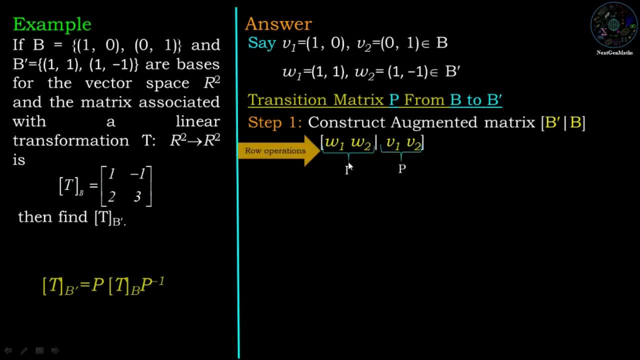 and apply row operations such that this first part convert into the identity, So V1,. V2 convert into the transition matrix, So W1 equal to 1, 1, 1. first column, W2 equal to 1, minus 1. second column, V1 equal to third column 1, 0 and the fourth column 0, 1.. 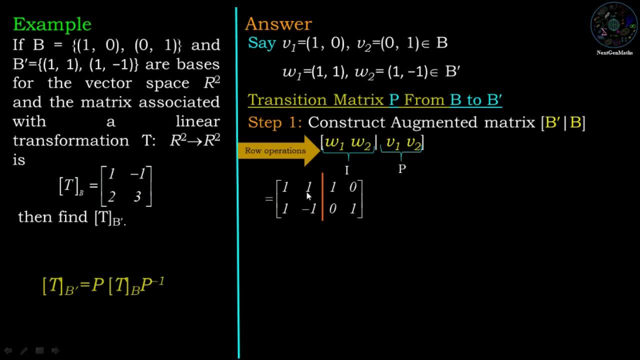 Now we try to convert first part into the identity matrix. for that we will use the row operation. So first row operation will make this entry 0.. So multiply first row by minus 1, add it to the second row. Then we have minus 1 added to the plus 1, 0.. 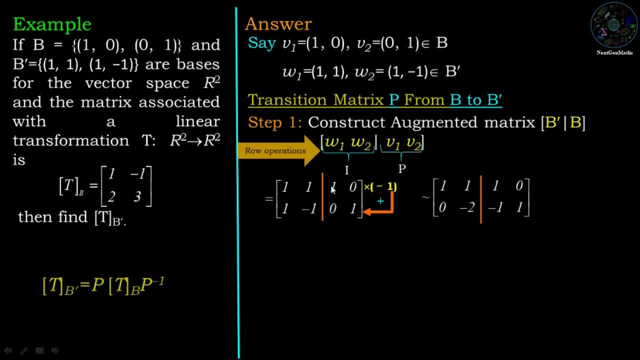 Then we have minus 1 added to the plus 1, 0. Then we have minus 1 added to the minus 1, minus 2, minus 1 added to the 0, minus 1, and 0 added to the 1, 1.. 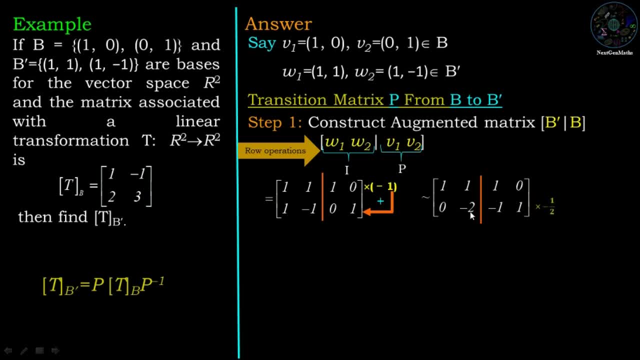 Now make this entry 1 by multiplying minus 1 by 2.. Then we have 0, 1, 1 by 2, minus 1 by 2.. Now make this entry 0.. So multiply second row by minus 1 and add it to the corresponding entries of first row. 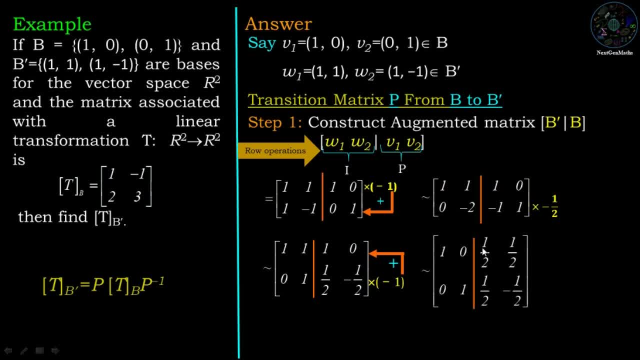 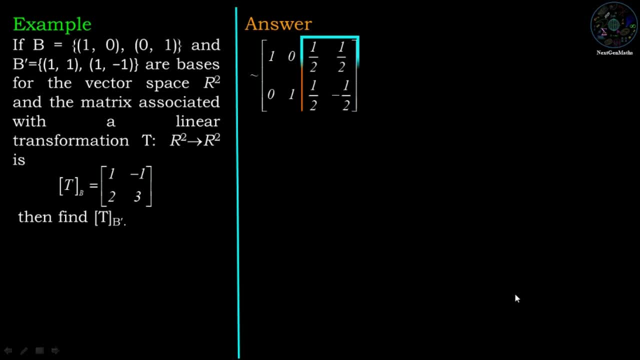 Then we have identity in the first part and the second part: 1 by 2,, 1 by 2,, 1 by 2 and minus 1 by 2.. Therefore the second part will give the transition matrix which is 1 by 2,, 1 by 2, 1 by 2, minus 1 by 2.. 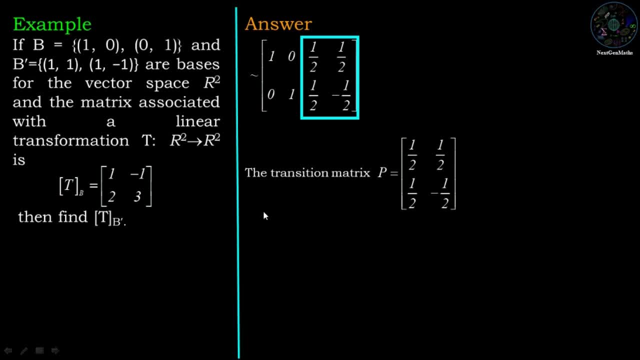 Now we have to calculate tb dash. So use the result: tb dash is equal to p, tb, p inverse. So this is p, tb and p inverse. Then we have final result: 5 by 2,, 1 by 2, minus 5 by 2,, 3 by 2.. 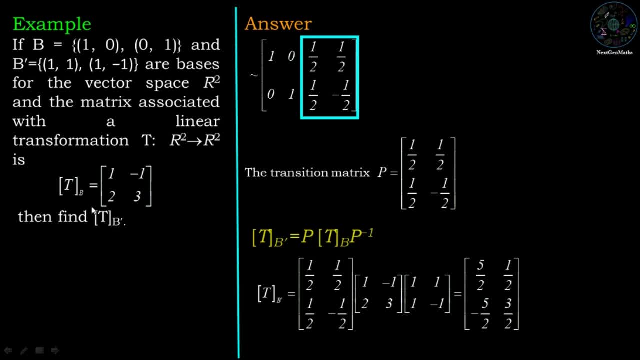 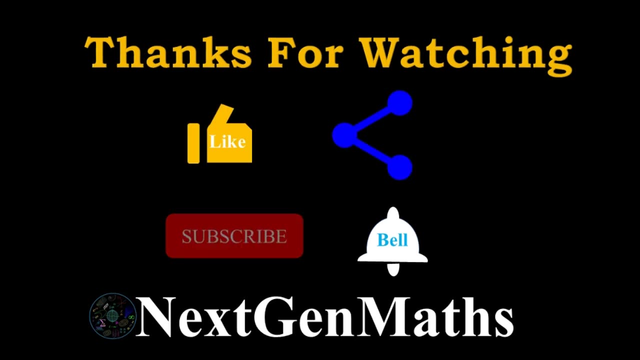 So this way we can calculate tb dash using tb. Through this result, tb dash is equal to p, tb p inverse. Thanks for watching. Like, share, subscribe and press the bell icon of NextGenMess. 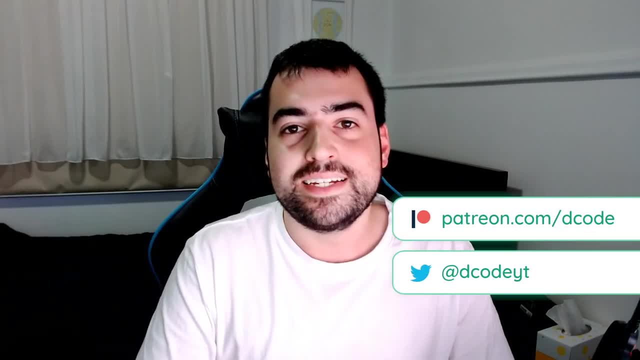 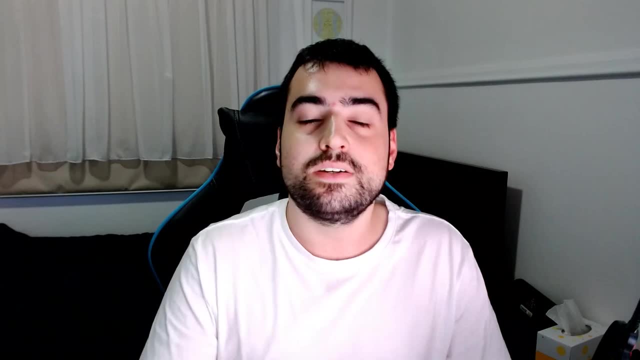 Hey guys, how are you going? My name is Dom and today we're going to be taking a look at the basics of JavaScript events. Okay, so today's video is going to be perfect for people who are just starting out to learn JavaScript, or you've got a bit of experience. 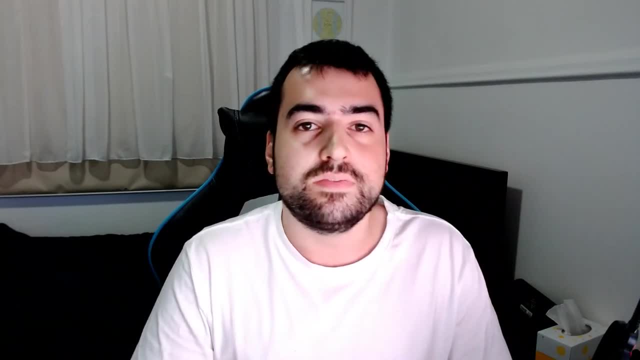 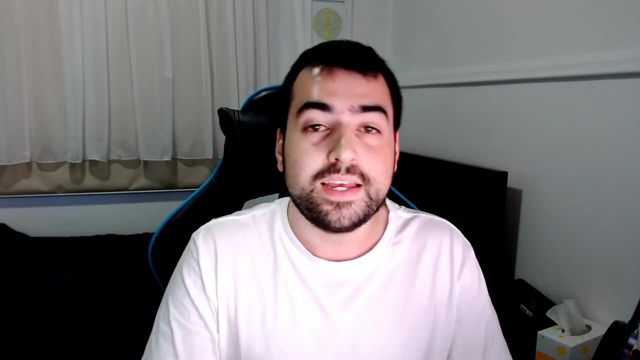 under your belt and you just want to get a recap on how the events work. Okay, so, of course, the first question here is going to be: what exactly are JavaScript events? Well, essentially, they're going to allow you to react to when certain things 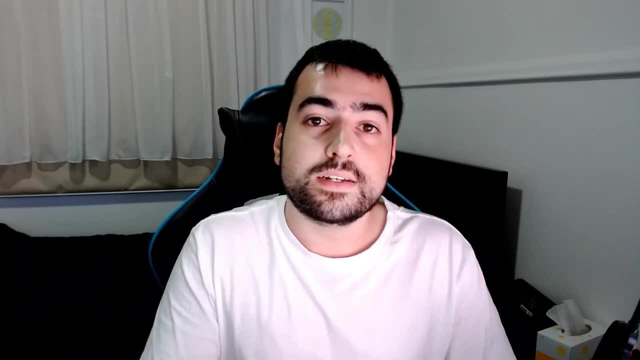 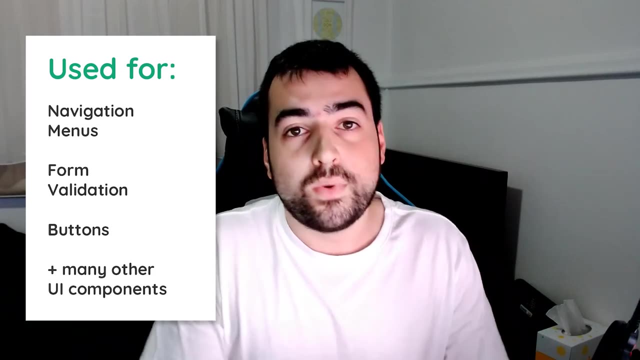 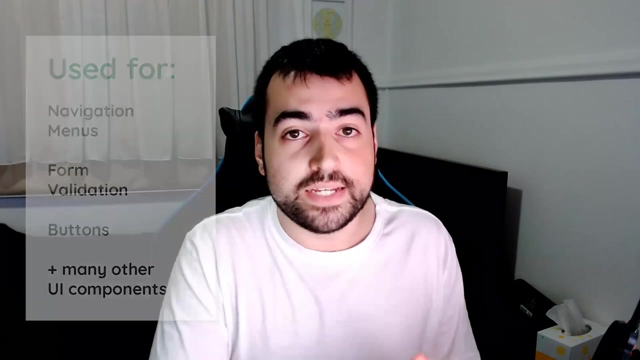 happen on the page. So, for example, when the user clicks on a button, I want, for example, a drop-down menu to show. Or another example might be: when the user clicks on a submit form, I want some sort of validation to happen. So basically, you have the event and then. 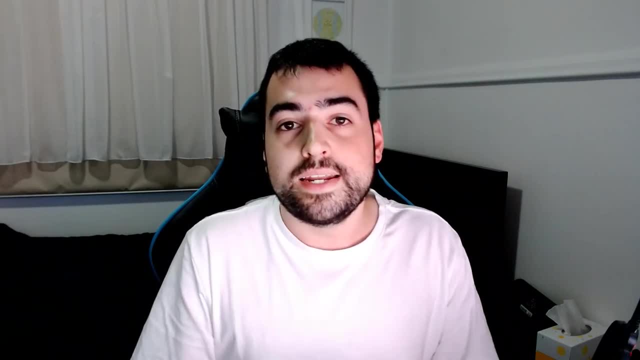 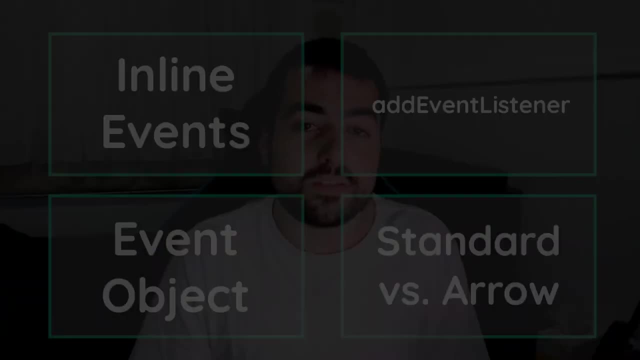 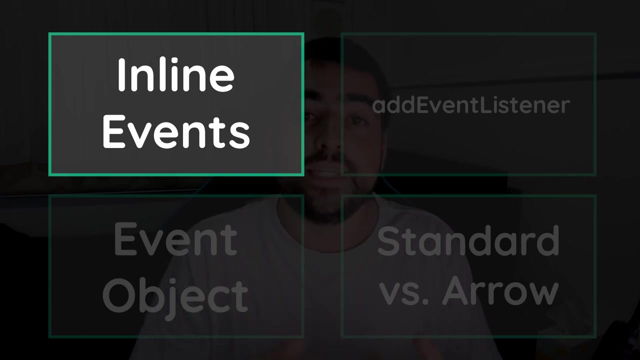 you have the action. So in today's video we're going to cover four main topics around the events to, of course, gain an understanding of how they work. So the first topic covered is going to be the usage of the very basic HTML inline events. Okay, so these are things. 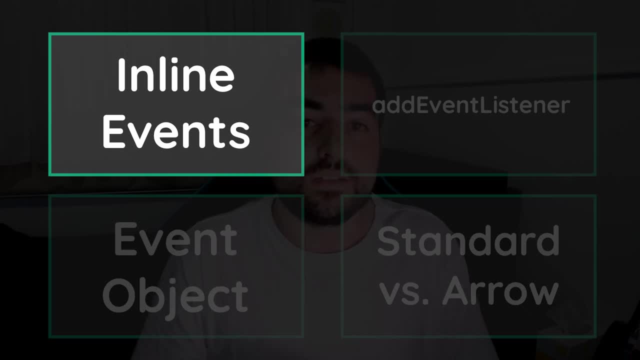 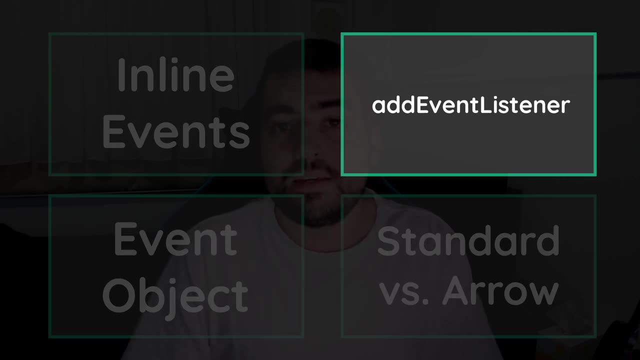 like your onClick, which you'll see on many beginner tutorials. The second topic covered is going to be the usage of the addEventListener function, and this one here is arguably the most important. The third topic is going to be the usage of the JavaScript events. So the first topic covered is going to be the usage of the addEventListener.